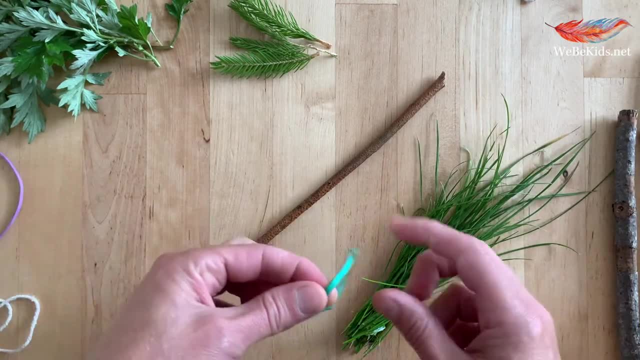 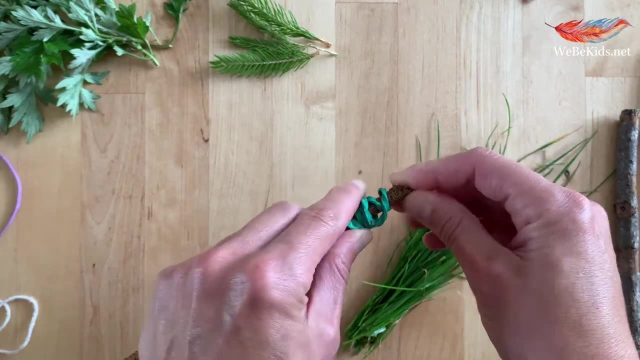 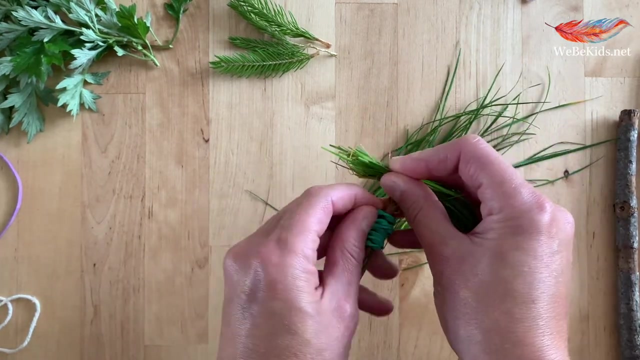 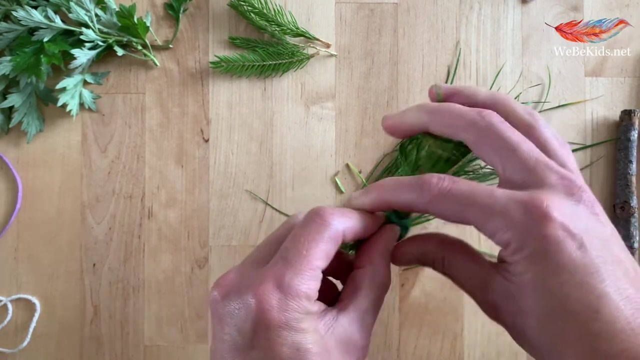 a bunch of grass And you're going to take an elastic band and wrap that around the tip of your stick like: so Leave a little bit of give so that you can take your grass in small bunches and you can lift the top of the elastic here and slot the grass through. So you have two points. 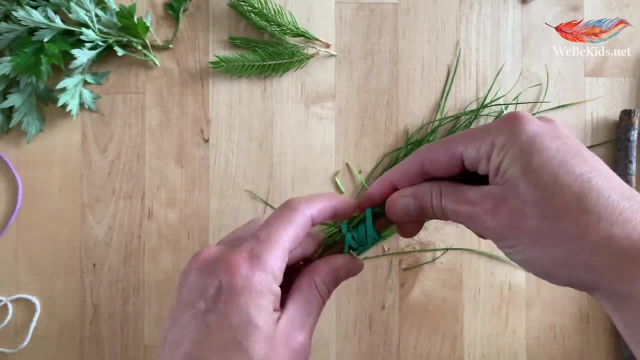 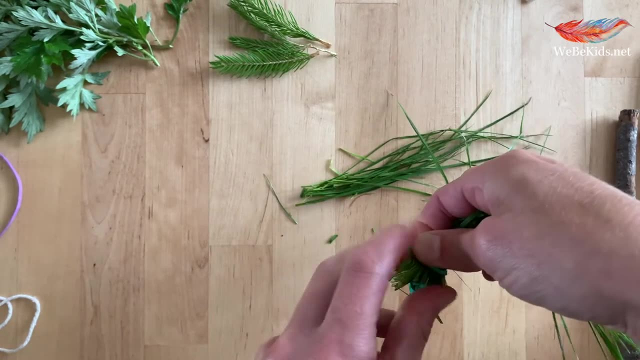 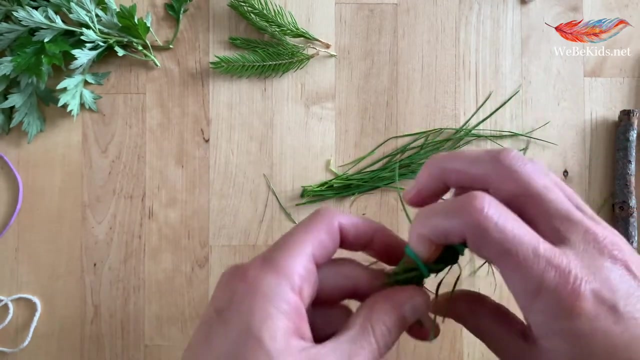 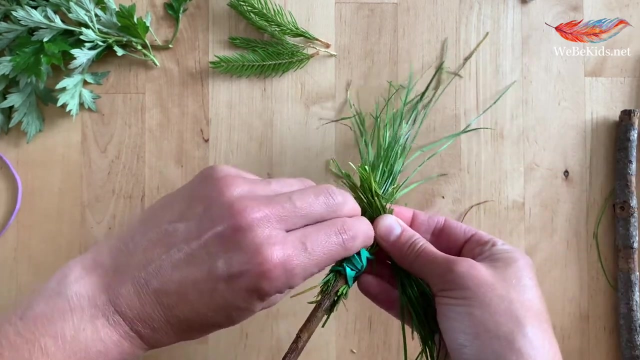 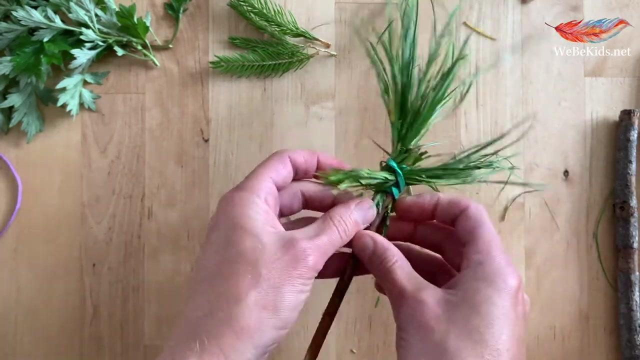 You can also slot it again with the bottom elastic And you can spread your grass around your stick. And I'm doing this in three sections- You can choose more sections than that if you would like. And my final section, gathering up the last pieces, securing top and bottom, just lining. 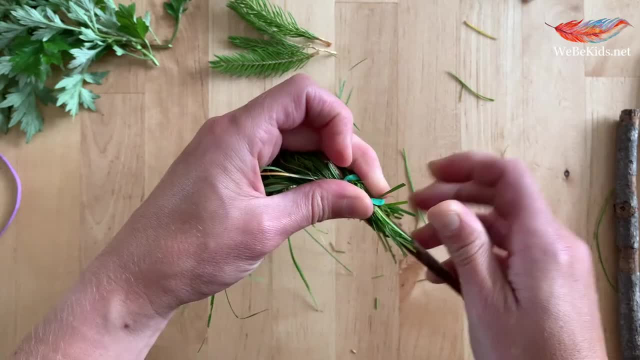 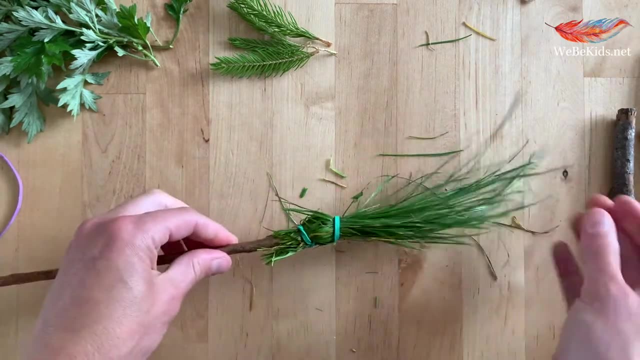 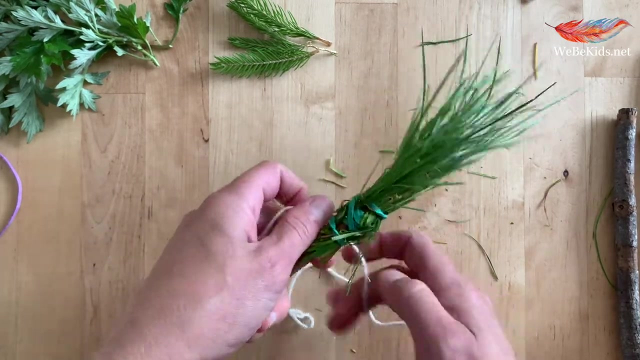 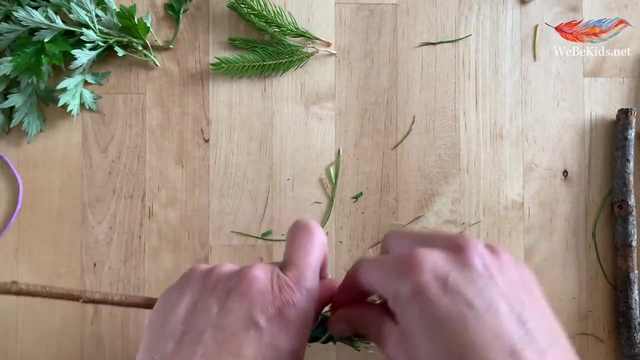 those up Now. as you can see, that is sufficient. You could just go with that. Or, if you're worried that some of these are loose, you can also take a short length of string or twine and simply wrap that over your chosen material. Then, having wrapped that around, just to secure, 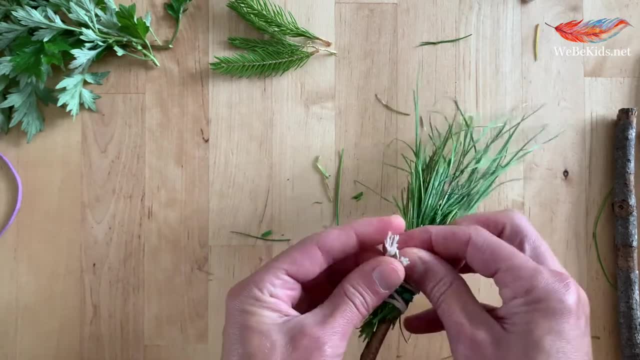 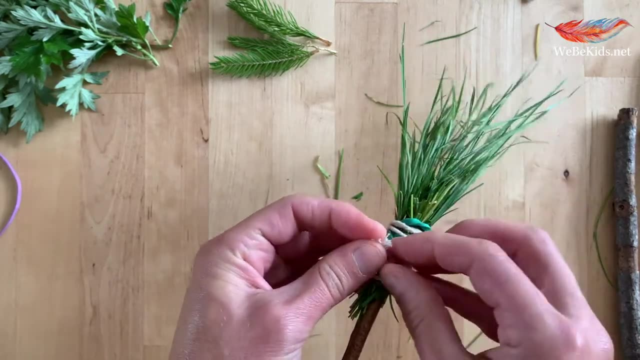 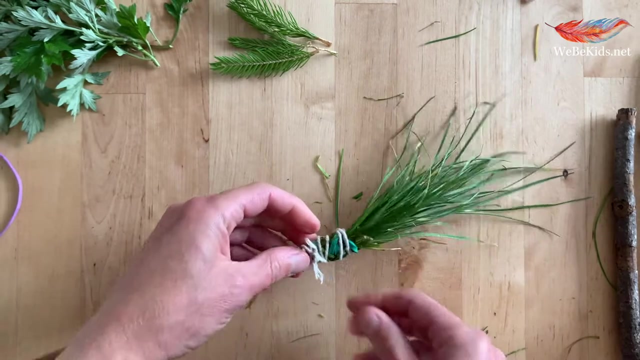 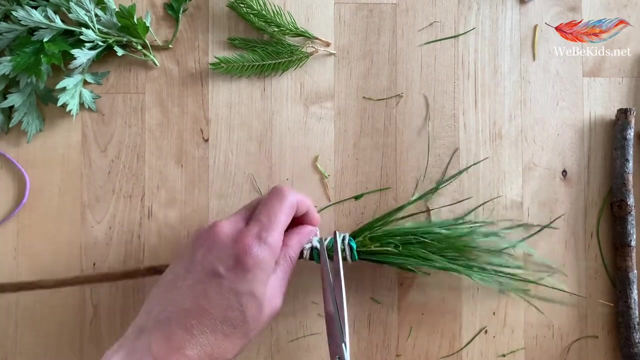 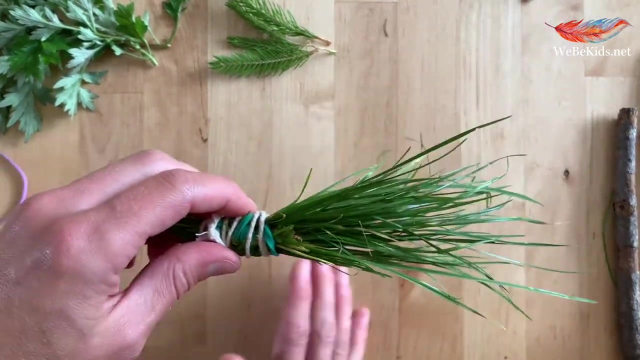 them all. you're just going to tie your ends Nice and tightly with an overhand knot And then, if you want to, you can also snip away any loose ends, And there you have a natural paintbrush. Now, if you're going to use a brush, you're going 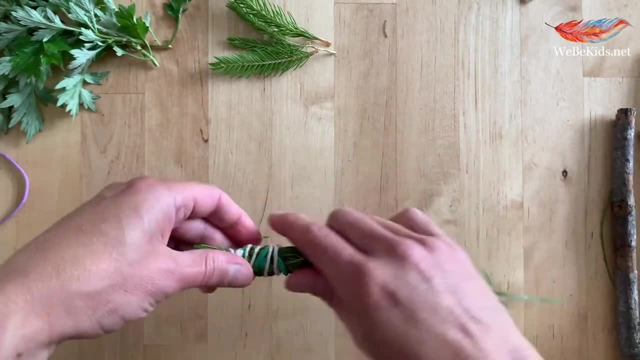 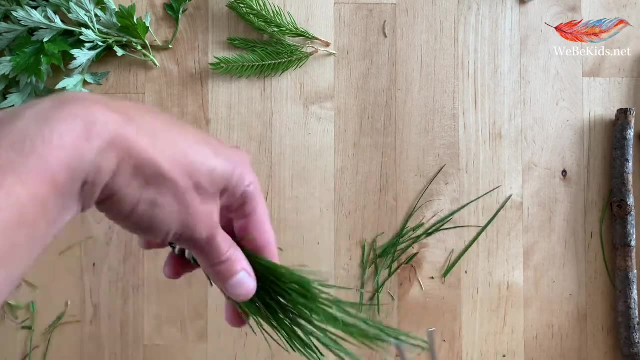 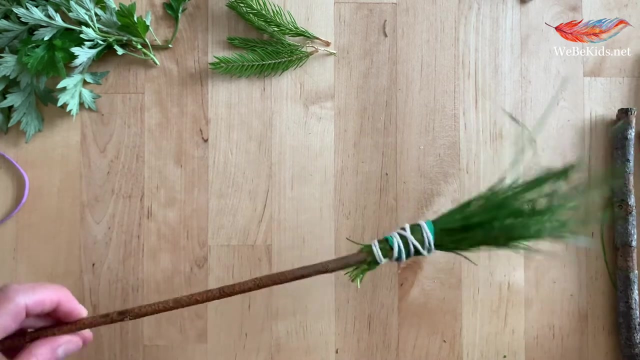 to want to use a paintbrush. Now, if you aren't happy with the taper or the length of your brush, the shape that it makes, you can also use your scissors to cut it into a shape. I'm actually not too unhappy with what I have here, But you can also snip them into the. 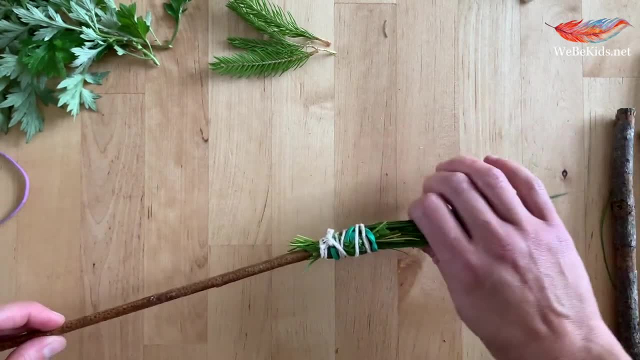 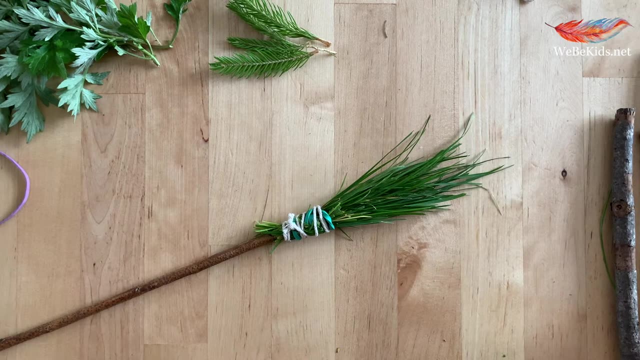 shape that you would like to have. And there we have our natural paintbrush ready for use on a large surface. Now remember: these paintbrushes aren't designed to give you great detail or accuracy. They are going to give you mark-making.